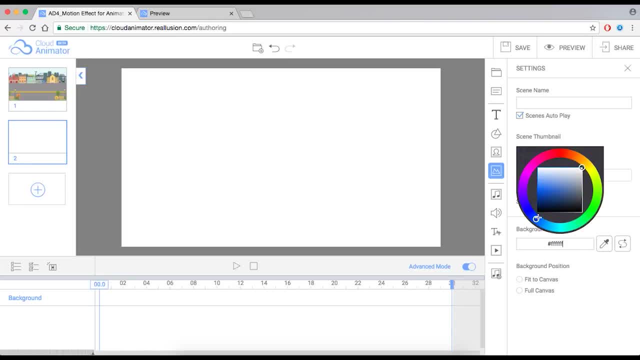 bring me to the background color of the settings, And I can easily choose a color that I'd like for that sky. Something bluish looks like a nice sky. I think that would look great. I like that. Okay, so what do we do next? Well, how about we grab some images and we start bringing 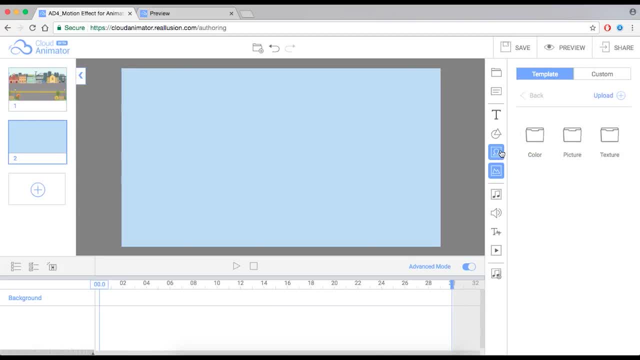 in these elements for the road and the city and whatnot. So I've already imported some of these. I'm going to go to custom here And I have my images. yes, Let me go down and I will simply start clicking on some of these assets. 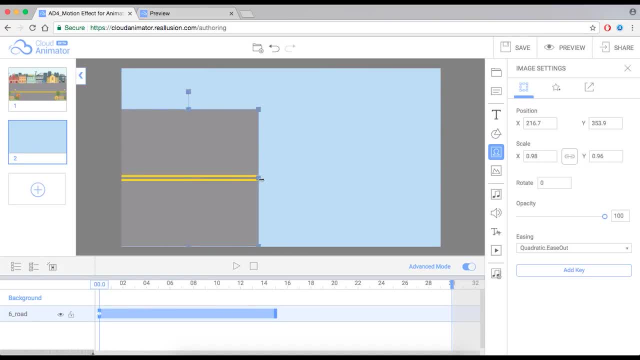 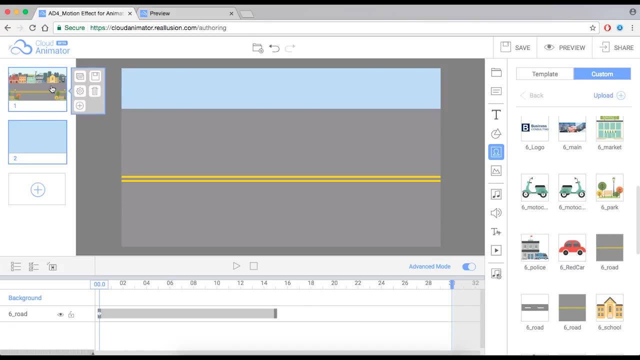 To import them, Okay, and I can stretch them out. I can do this manually, as I'm doing it right now, or I can play with scale. I can do this, if I'd like to, to give it specific values. So we've got our road. Now what we need is the city, that background city here. 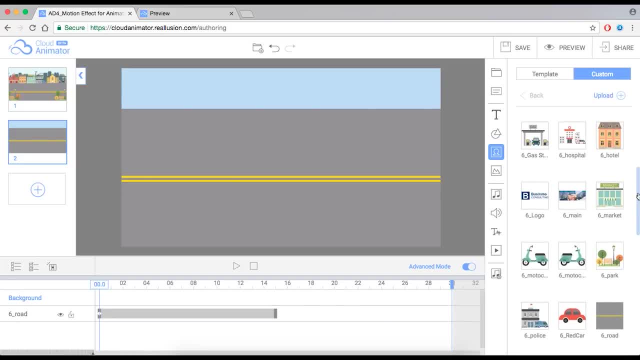 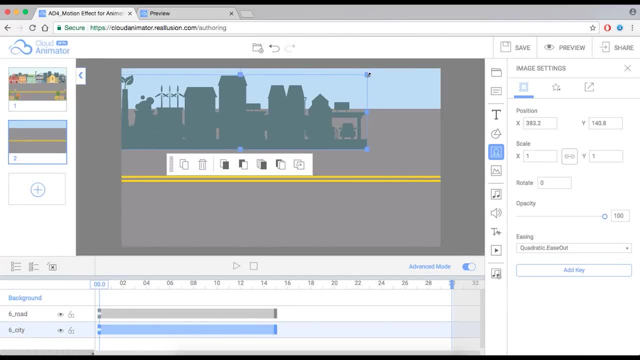 So we have that element also, this PNG that I uploaded before, the city one here And I simply have. I can arrange it, but let me give it a scale of 80%, Okay, And we're going to bring this up a bit And I think it should look okay like that. Yeah, that's not bad, Let me bring. 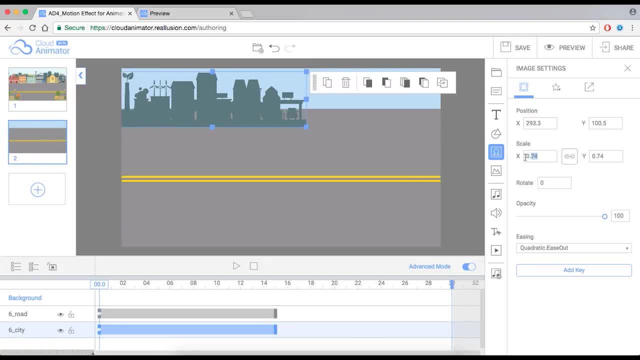 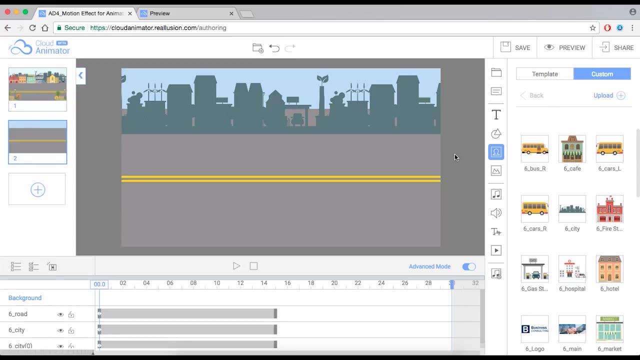 it. let me make it smaller a bit, Or let's leave it at 80.. Okay, So I can go in and grab another one, or I can duplicate this, which is what I always recommend. You don't have to invent the wheel. If you put in that effort, just duplicate it, And it's very, very easy. 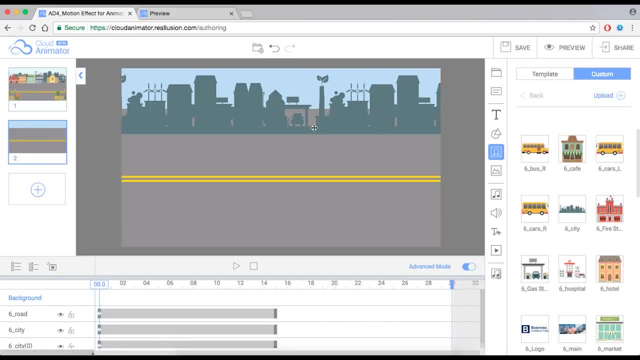 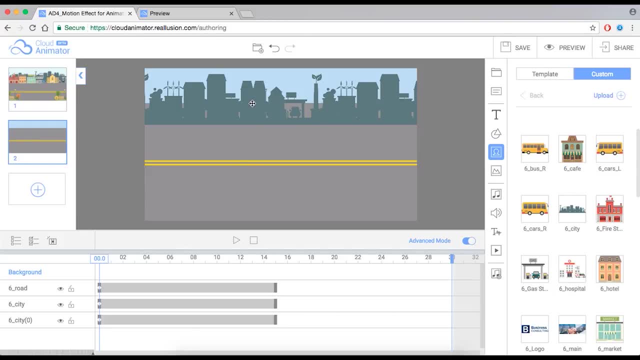 to play with that later on. Okay, So we've got this background and I don't wish to play with this any longer. So, in order to avoid making any mistakes while dragging stuff on top of it, we're going to lock this down. I'm going to lock the road and lock the two. 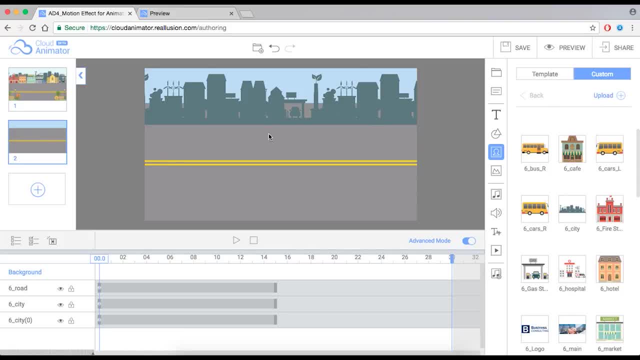 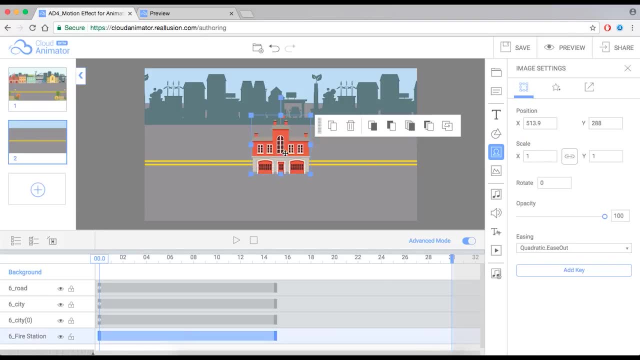 city scenes in the background. Okay, And now what we want to do is start adding these buildings. So, as you guessed for the buildings, it's very simple: I just drag and bring them in. I can scale these again. Give me 80%, And because the X and Y are linked, so the Y will. 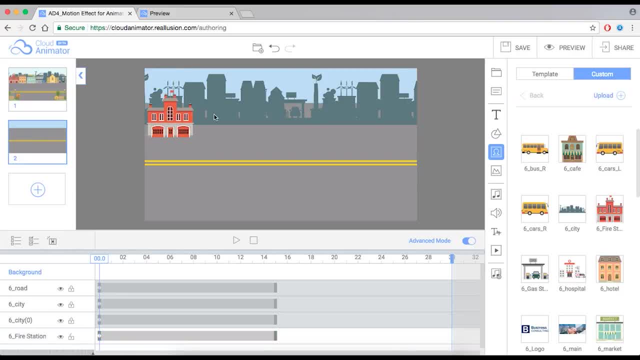 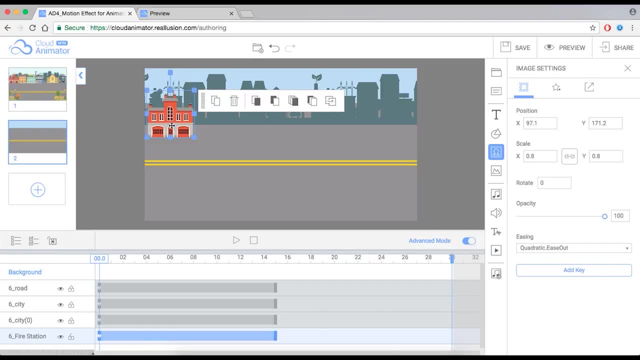 also be 80%, And that makes it a lot easier. So here, what I like to do is, instead of bringing in another asset, there's a little trick. I can actually duplicate this. bring it to the side, Okay, And then I could replace it. I want to replace this with another image, So what I'm doing? 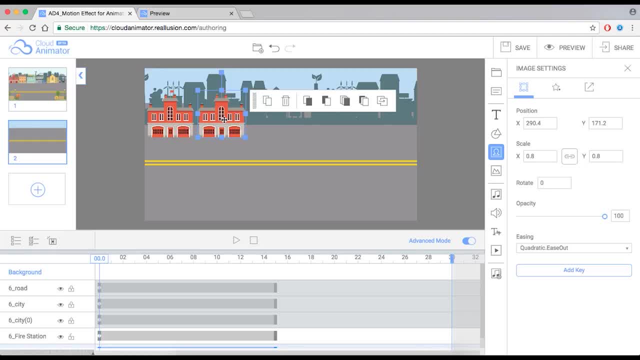 here is that if I copy this, at the same time I can also copy the effect that I drop into this object. So I'm not going to show that right now. Right now I just want to keep that size and I want to keep that position. I want to keep those values inside my element. 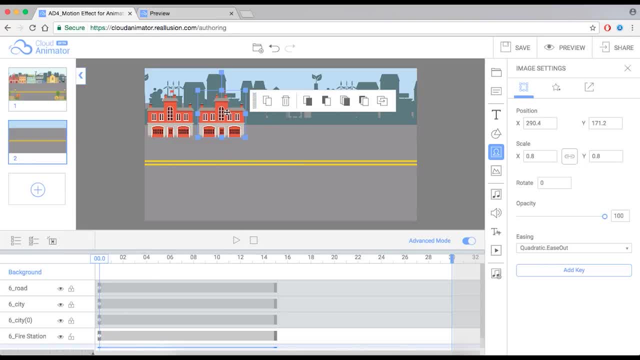 which are saved inside the keyframe. Okay, So if I want to replace this with another object, I'm going to drag and bring it to the side. Okay, So if I want to replace only the visuals of that element, I can go up here onto the side. 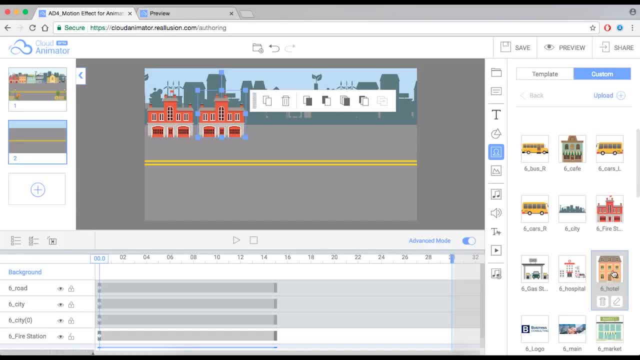 It says switch to image, And then I can go in and I can select a different image. Okay, You see that. And then if I want to make sure that I'm using the correct proportions, the original proportions of that new image that I'm bringing in- I can right click Whoa. 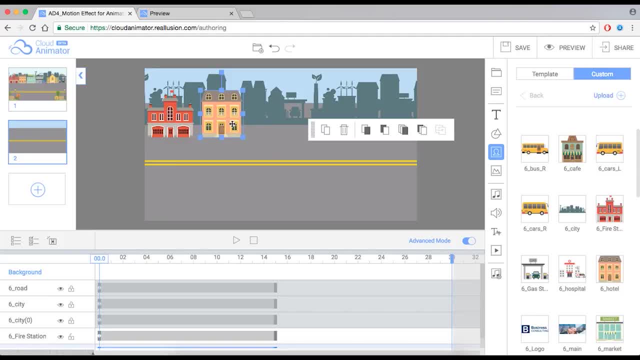 hold up, Right click and click fit, Okay, And that'll ensure that I am bringing the original proportions of this new image, of this new prop that I have. All right, Let me squeeze these in and let's do the next one. I'm going to select it, I'm going to 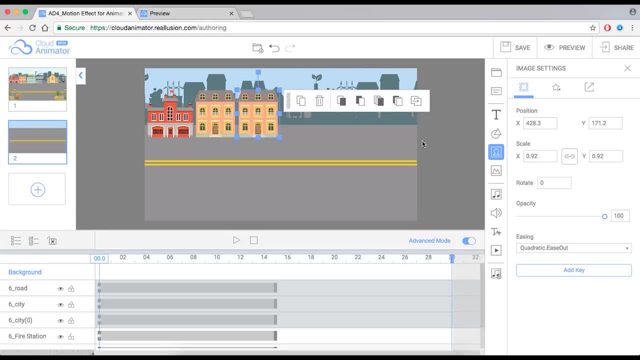 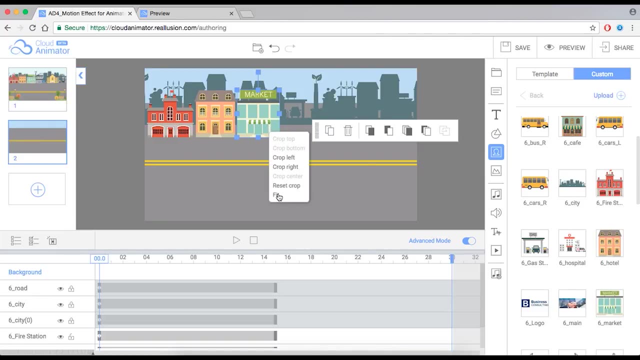 duplicate it, bring it to the right, And then we wish to replace that image, right. So let's replace. switch to image and let's find that other building. Let's choose the market. All right, That looks good. So I'm going to right click. just hold that right click, then fit. 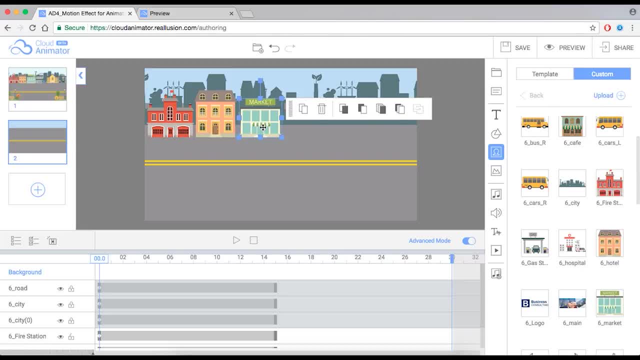 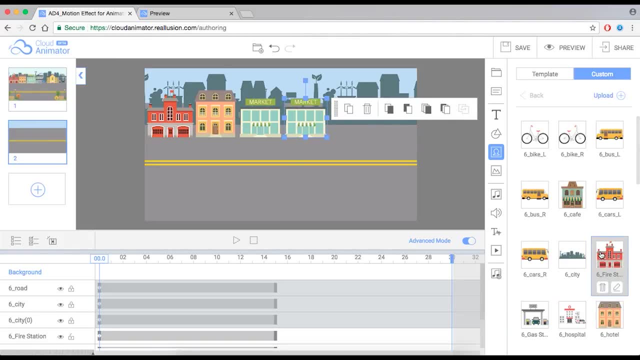 That'll ensure that I'm going to get the different proportions Okay, And then, if I want to do, ensure that I fit the right, the correct proportion of my image, and we're gonna do this repeatedly with the other elements. what's the next element that we? 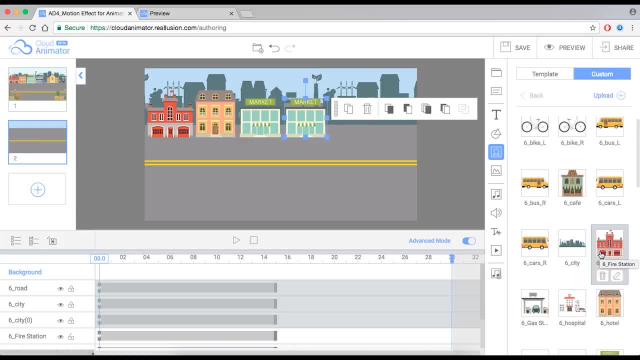 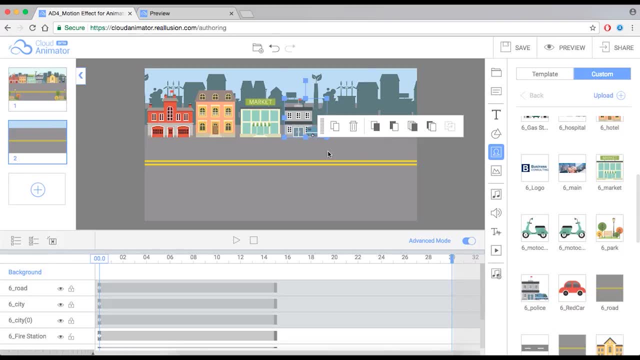 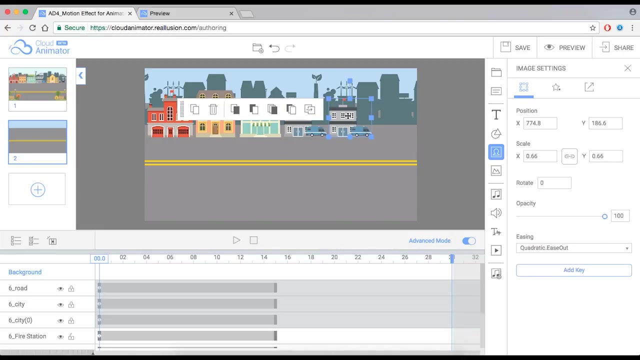 had. I think it should be some gray building hold up. I'm looking at the image here on the left of police station. yes, there we go. police station, right, click and fit. okay, and I make sure that we have that right proportion. all right, let's do that again, bring it to the side and then, now that we have it, 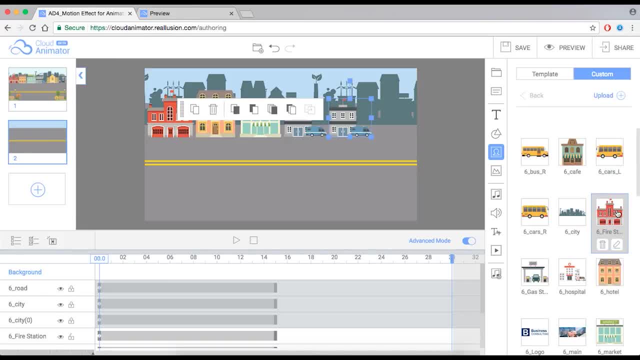 selected, I'm going to replace that image and this time around I am going to choose. I think we have a church in here, nice little church. where are you? or I'm sorry, it's a school, so we have the school right there. let me move this a. 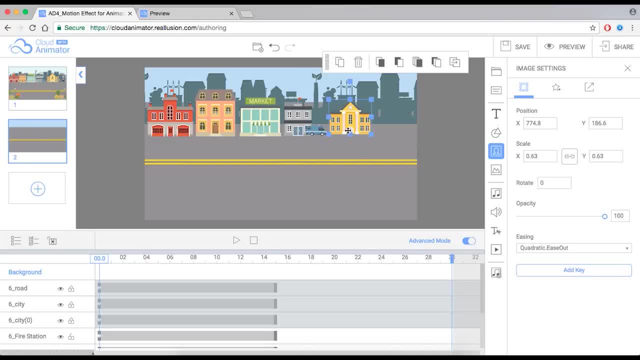 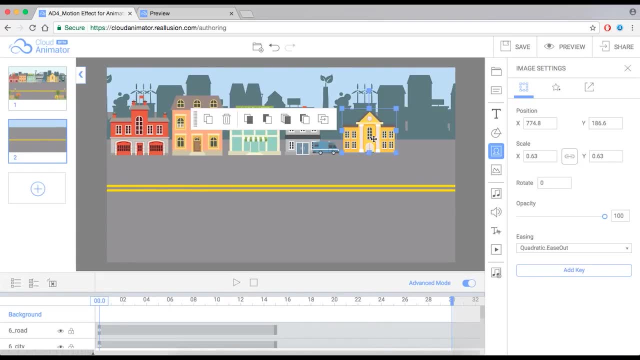 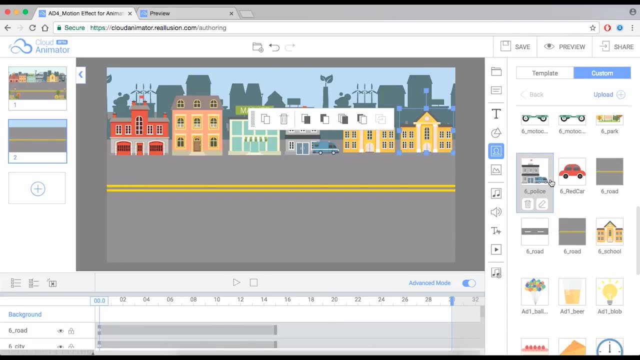 bit and fit, and that looks actually pretty good. I like it. you this down a bit, all right, so we're almost done. I'm gonna duplicate this one more time, bring it to the side and this time we're gonna replace this one with- you guessed it- the police station. I think it is the police station, or is it? 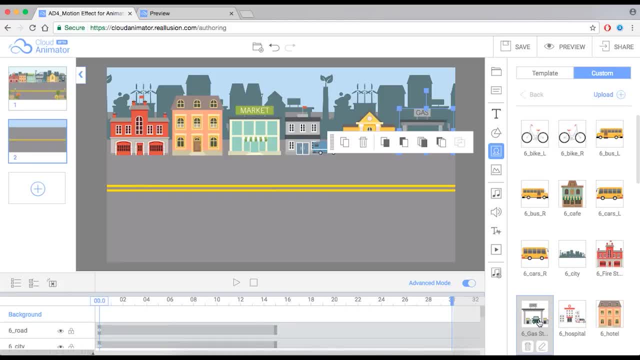 the gas station. I think it's a gas station right there. boom, we have that gas station, and then finally hold the right button on it fit to make sure we have that correct proportion. great. so now we have all these items here. let me bring that right there and we are ready. so but what about? 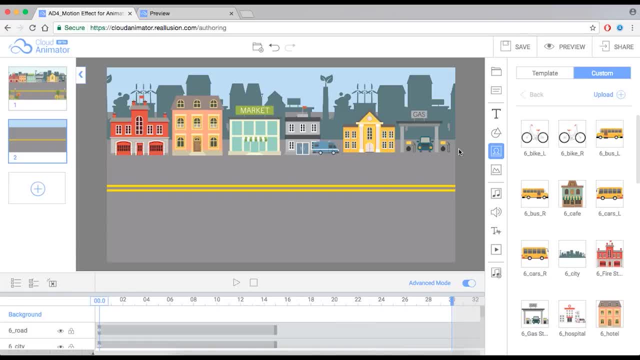 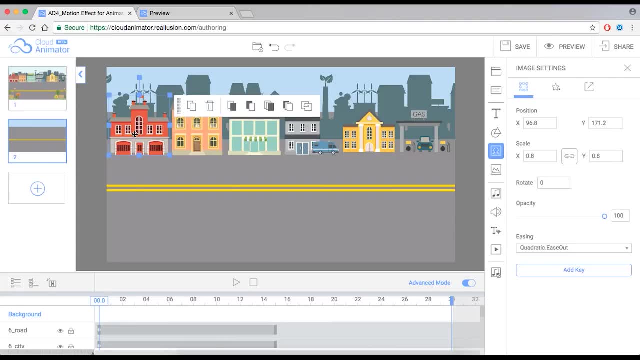 if I wish to add the effects, if I wanted to add the effects to these, to have them pop up. so I can obviously do this manually each time. right now- we're tonight- when I have this here, I can start adding the motion effects and I can copy that. and every time I copy it I'll be copying the scale, the motion. 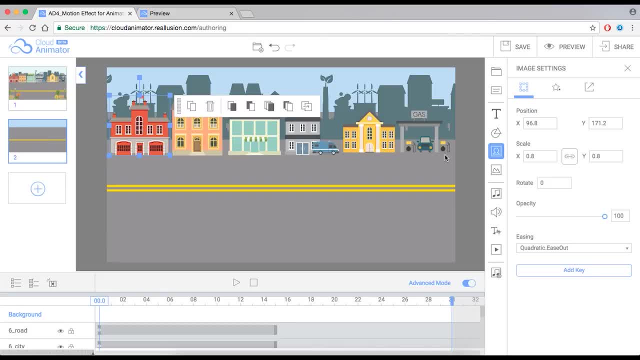 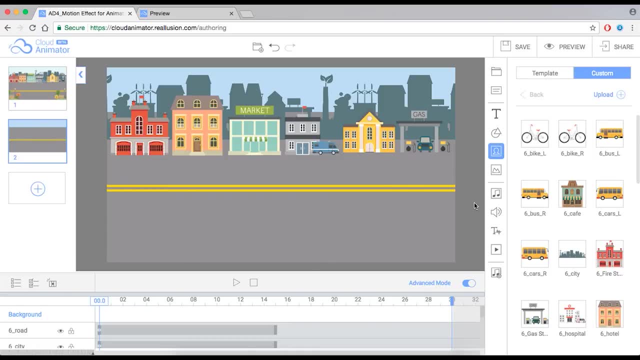 effect the position, and that will translate to each and every item of the and every element that I'm adding, but I'm gonna do that until the very end. right now, what I want to do is I want to fill up my screen with all the the elements that I need. so let's go to park and we're gonna bring this in. let's give. 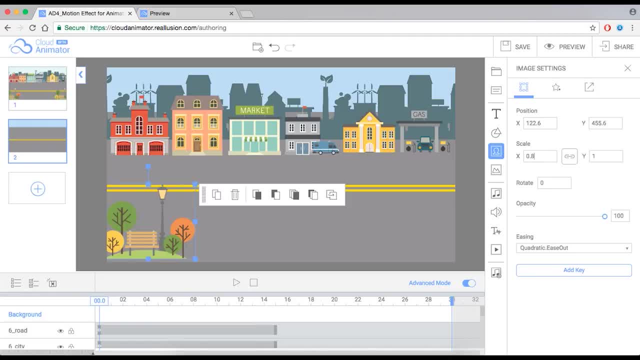 this an 80% also, so that would be 0.8. yep, and squeeze it in there, yeah, something like that- and duplicate this puppy, bring it to the right and that looks okay. I like that, okay, great. so what else do we need in the scene? we? 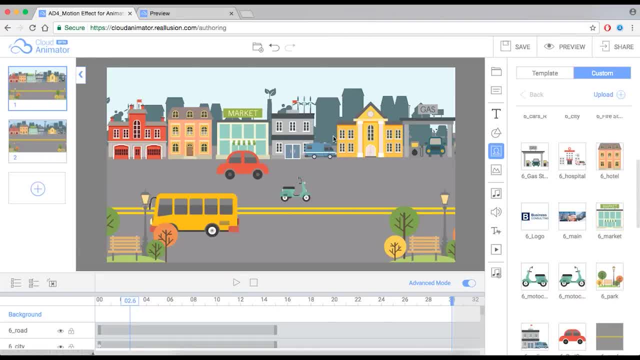 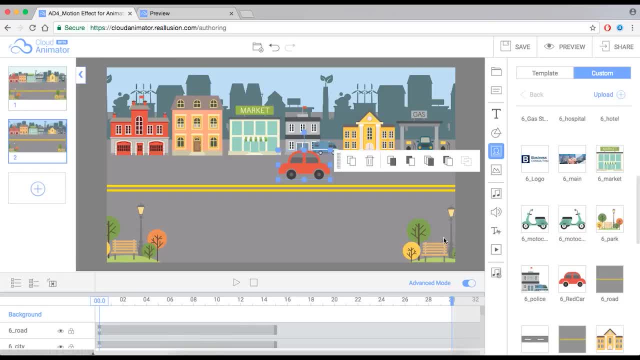 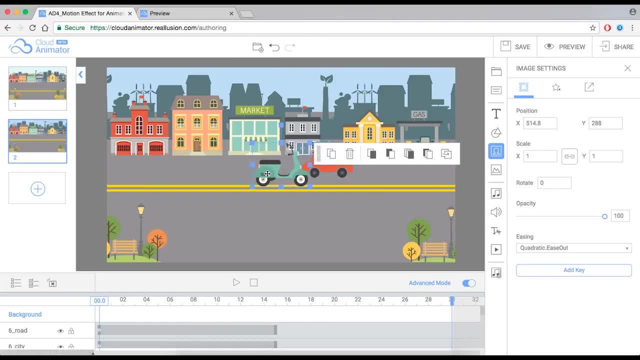 I just click, we have it in. great, what about that motorbike? that motorbike is going in a specific direction. I think it's this one here. oh, not the car, the motorbike like that, and I can scale this down a bit just to make it accurate- per. 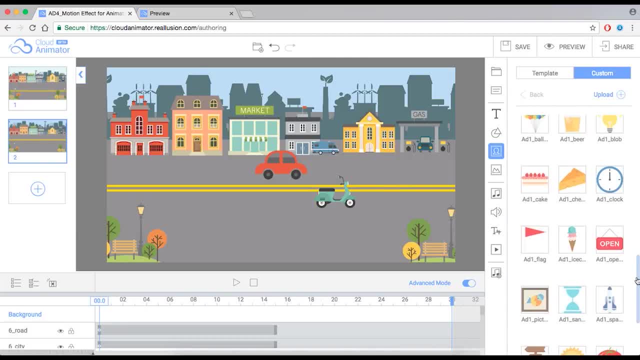 se, what else do we need? we need that bus, that bus, that little yellow bus. here we go. so we're gonna have this bus here facing towards this side now, obviously, because I pulled in this bus after I dropped in the park, it's actually trampling that park asset that we have. 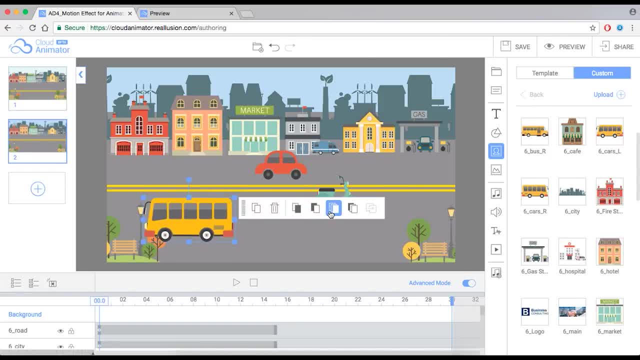 so what we can do is just make sure that you push this backwards. I can bring to front or I can ascend to back, but not all the way to the back, because then you'll place this behind the road. I don't want to do that, I just want to. 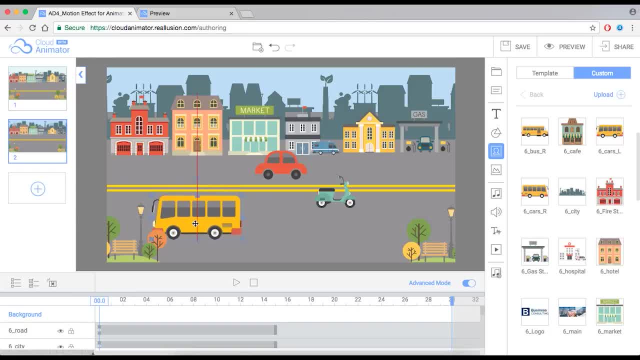 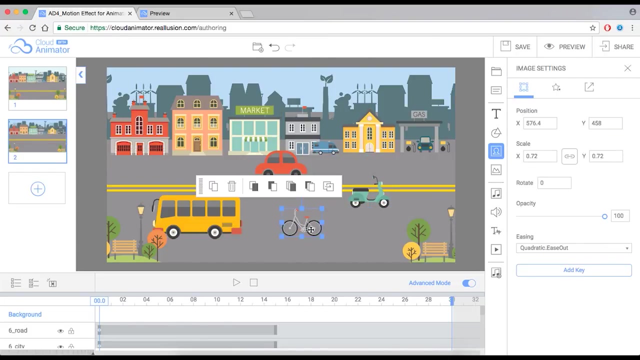 send back until it's behind that park, okay, and I think, just like that that'll look nice. and then, finally, we need our bicycle. where is our bicycle? this one, and we have our bike. let's adjust the size of our bike and we can bring it here, or we can move it to the other place. let's move this one here and 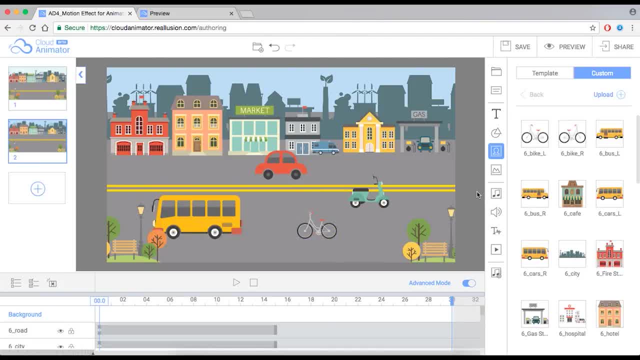 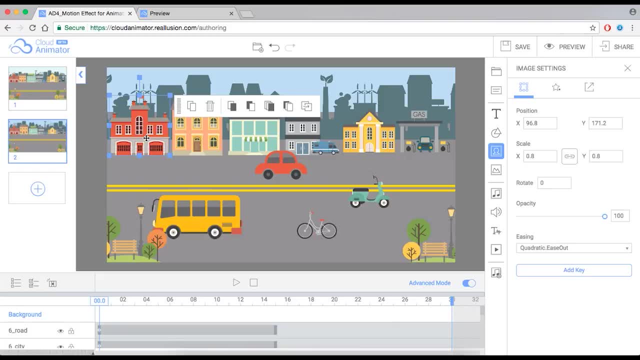 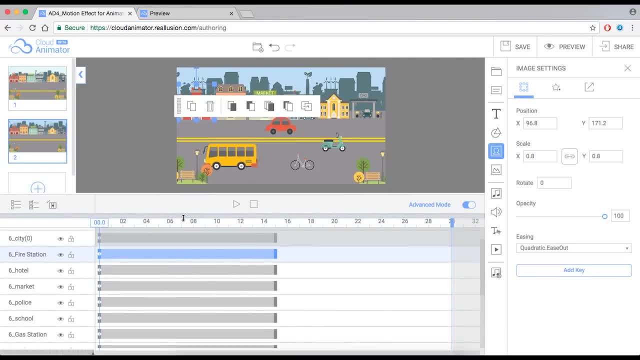 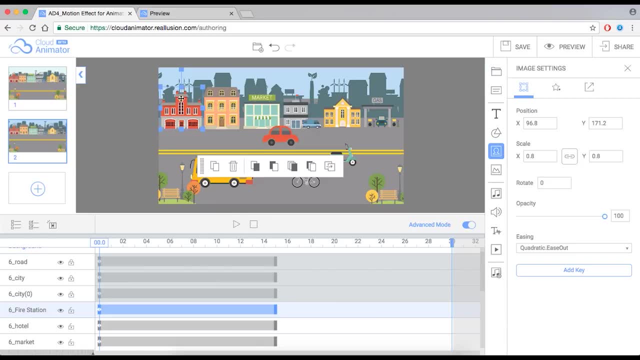 buildings. so I want to drop in some motion effects to that, to those buildings. so I'm gonna work first of all with the fire station. that's the first one and we have it selected. I'm gonna go to motion effects and then we have several motions that we can choose. let me just hover over. you scale this up. 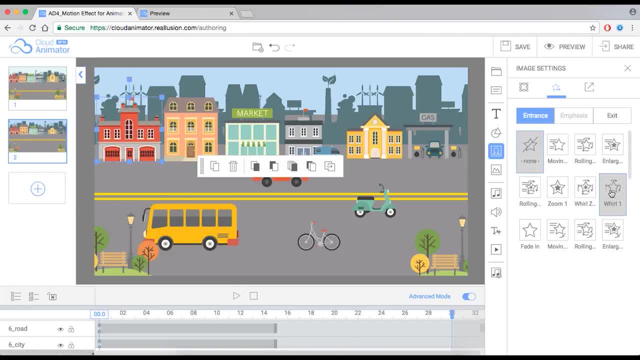 so you can see we have enlarge, we have whirl- remember that I'm. I want to work with the entrance ones. let me scroll down here a bit. we have this move- yeah, it looks okay. but for buildings, I want them to pop up right, I want them to to grow, sort of. so I believe that we have a pop-up effect. 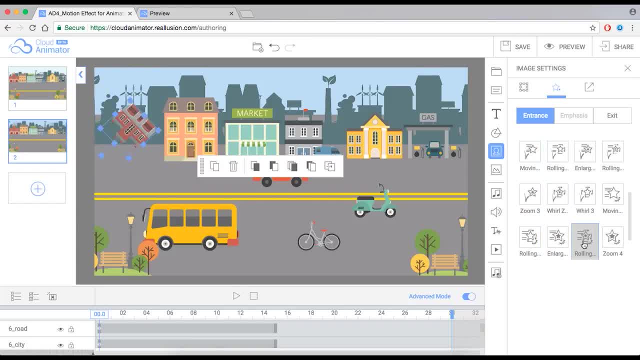 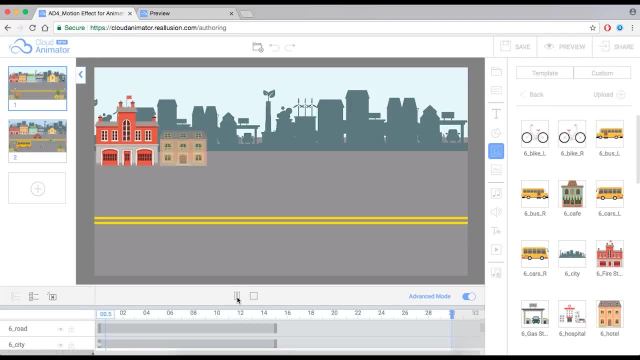 here somewhere, and large, no, rolling, no, let's see what's the effect that we had at the beginning here, see, they're all like growing from the ground. so that's a type of effect that we want. so we're gonna go ahead and go ahead, and go ahead, and 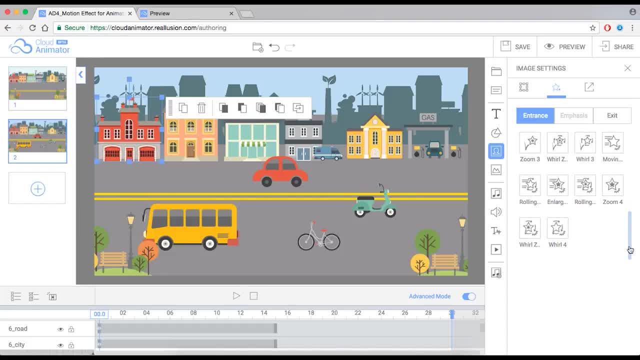 go. we just have to go all the way down until we find it. I believe this should be. what effect is this? let's try moving. well, actually, moving here doesn't look so bad. let's go down here. this one boom. I think this could work. so let's select. 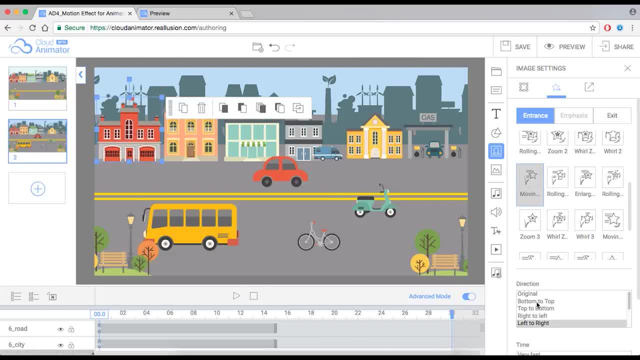 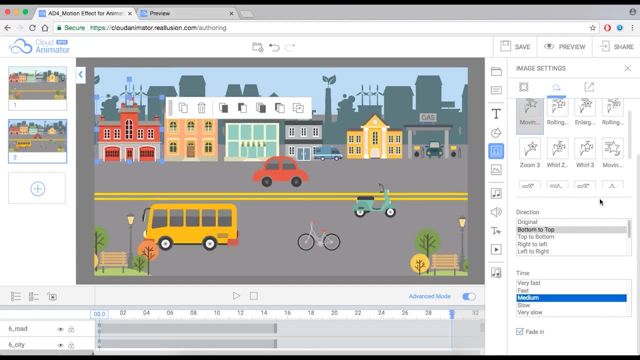 that one, and then we're gonna choose bottom to top. oh okay, I think that should look okay. let's do that medium boom. okay, and yeah, that could work, that could work. let's see enlarge, that could work too. let me see that one and do bottom to top. yeah, we can probably choose. 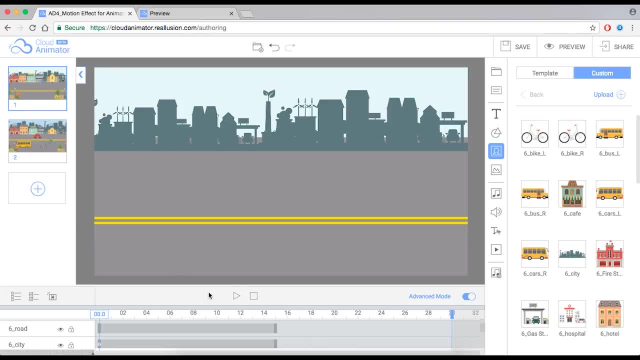 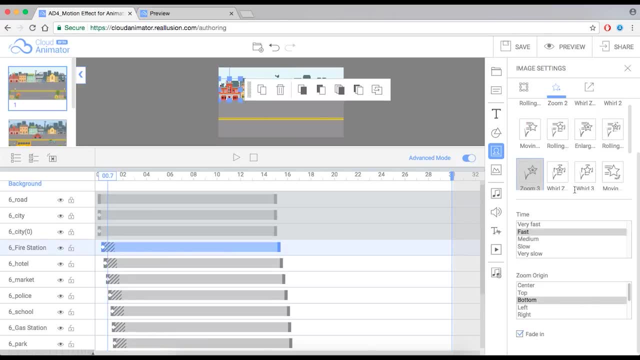 that I believe that if we go inside we can also, if we go into the original one, we can try to see the name of that first one that we were using. this is called a zoom see zoom zero three. so I think that, kid, we can use that zoom three and then 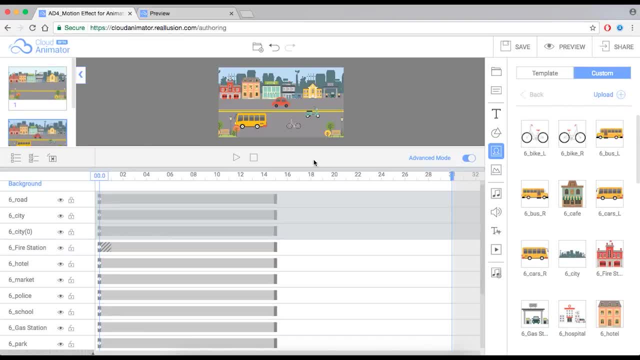 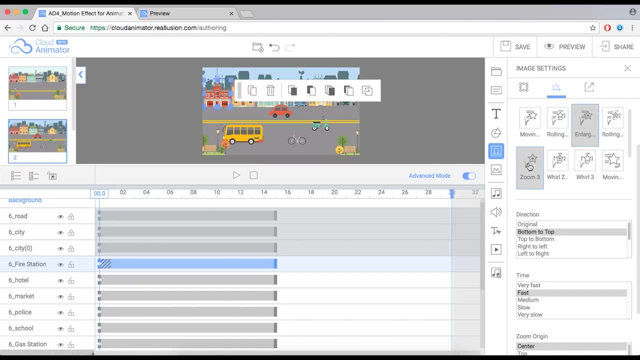 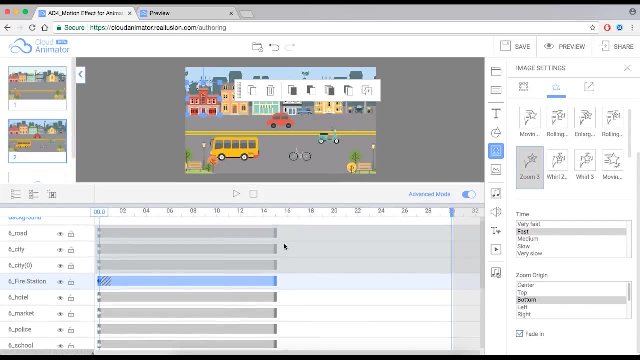 zoom in. I think that was the secret right there. so I'm gonna go in and we're gonna select a zoom three. we're gonna choose fast and we're gonna bring it up from the bottom. perfect, that's the one we want. see that effect? well, yep, that's the one we want. so I'm gonna repeat the same. 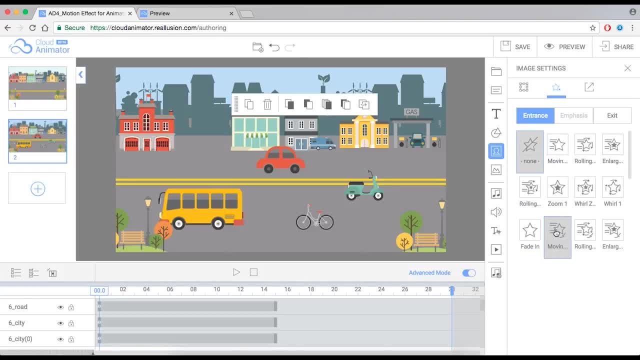 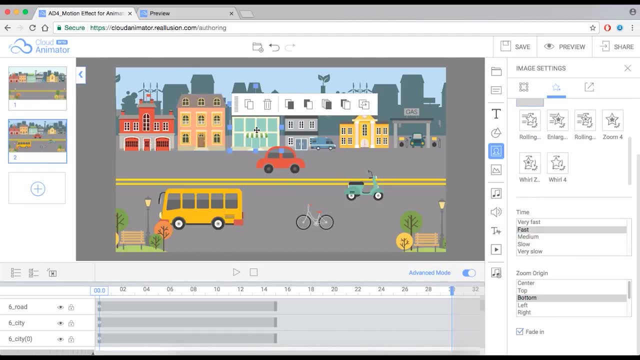 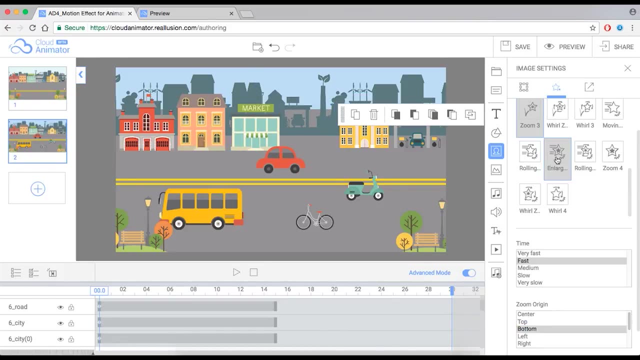 thing. for everything else, I'm gonna go to zoom three. we're gonna do this, I think, fast, and this is coming out pretty quick. the next one is gonna be the pull coming from the bottom. Now notice that the advantage of just copying things is if I wouldn't have to do this for each and every asset. 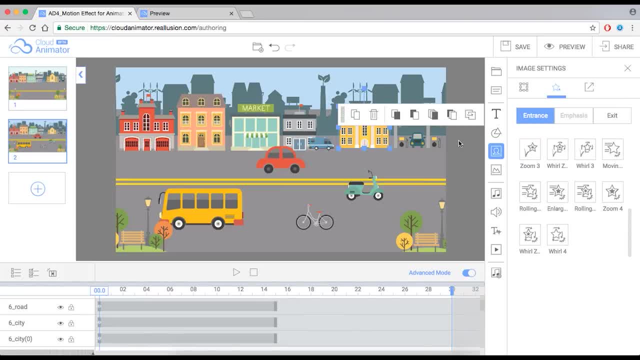 If I were doing, if I would have just copied the first one, drop in one element, scale it, position it, drop in an effect. then I can just copy paste over and over again prior to replacing that image, So I don't have to go through all this process. 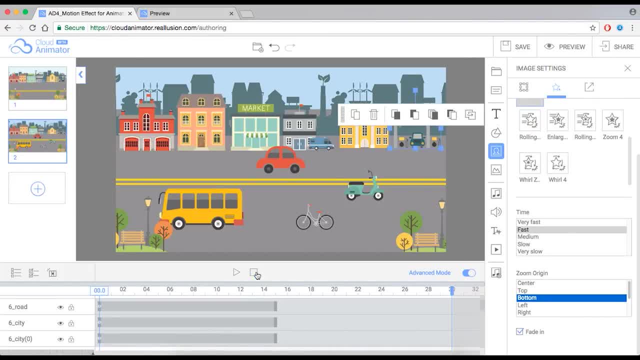 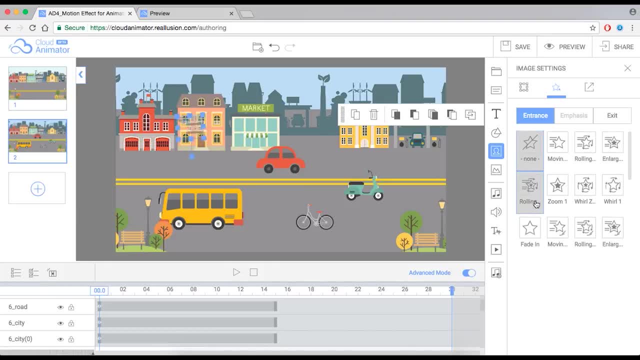 every single time. But of course, this is a tutorial and we are learning, So oh, here we go. We're missing one, which would be that one. So this guy should be zoom three and bottom to top. Great, that looks nice. 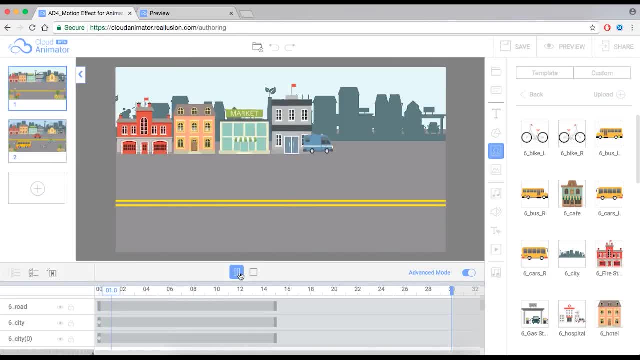 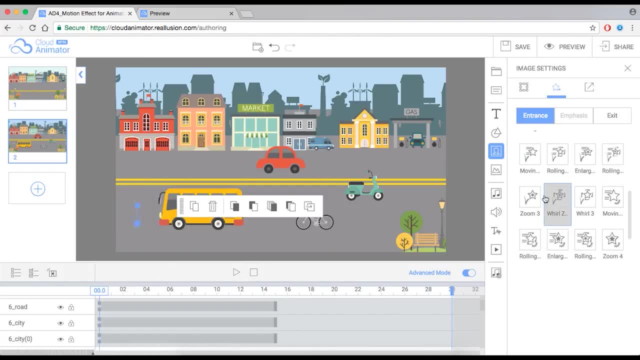 So let's go for the next one. Let's see what else We want: the park, the park. We want that to happen with the park also. So let's go. we know which one we need. Zoom three Fast from the bottom. 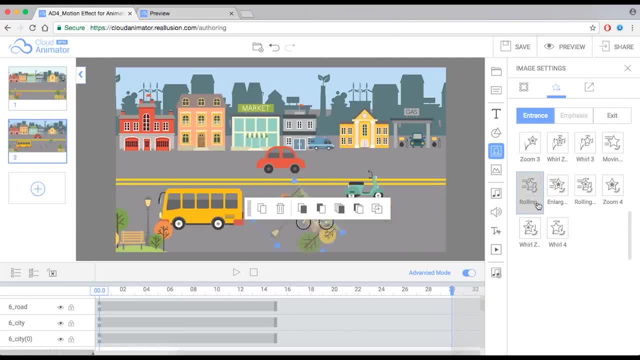 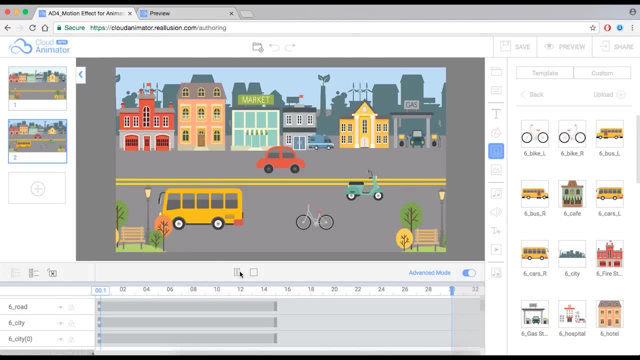 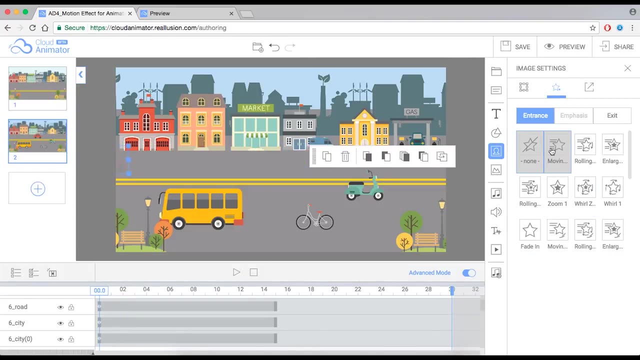 Thank you. User will also get the zoom three treatment with the zoom origin from the bottom Great. So if I play this back, boink, they all appear All right. so now it's just a matter of playing with the cars, with the vehicles. 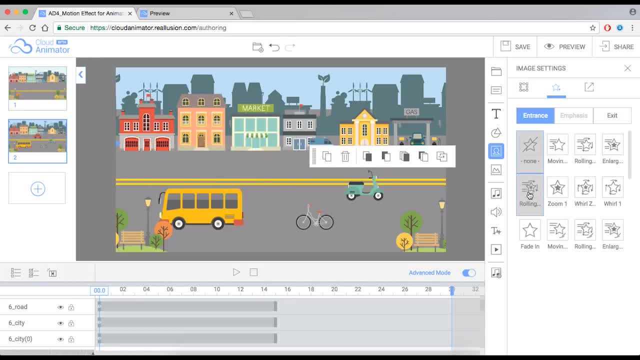 So for these, these are pretty simple. I can choose moving rolling fade in, but I want something with an elastic effect like this one. Moving this is very nice, Boink, okay. So I'm gonna have this one come in from the right. 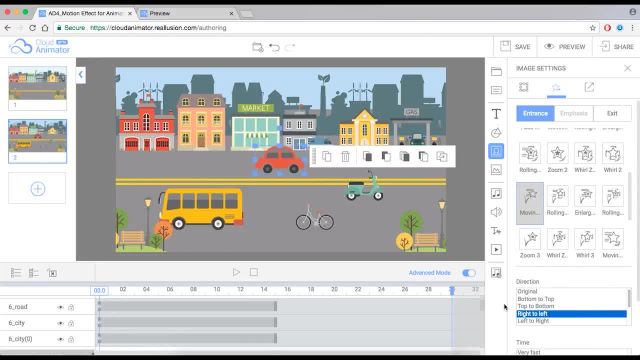 So I'm gonna select that and I'm gonna choose right to left, Okay, and I'm gonna choose medium, yeah. So then I'm gonna go to the motorcycle. This will do the same thing, but I want it to come from left to right. 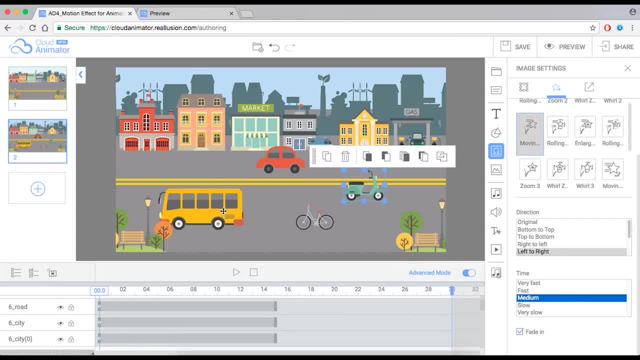 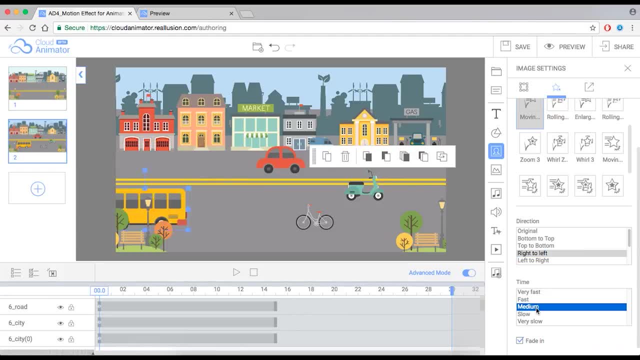 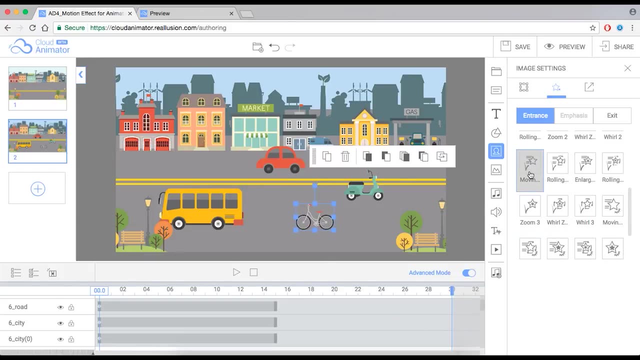 We have medium also, Okay. and then let's go to the bus. same effect, Moving, and this will come from the right to left. Let's choose this medium. And finally, the bicycle, too. Let's choose moving, Um, bum, bum, bum. is it moving? 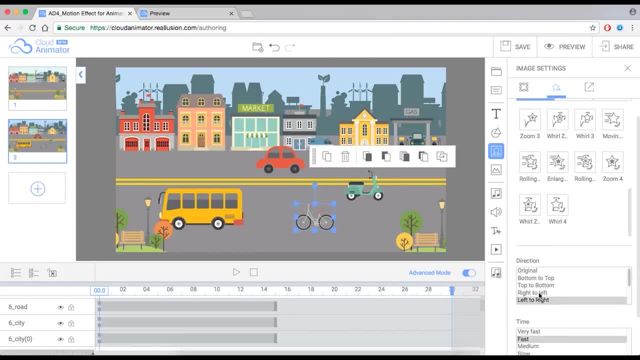 I'm sorry. yes, it is moving, and right to left, I think. See, moving right to left, All right, and let's do this medium, All right, and let's do this medium, So let's see what we can get. So let's go back here to the model. 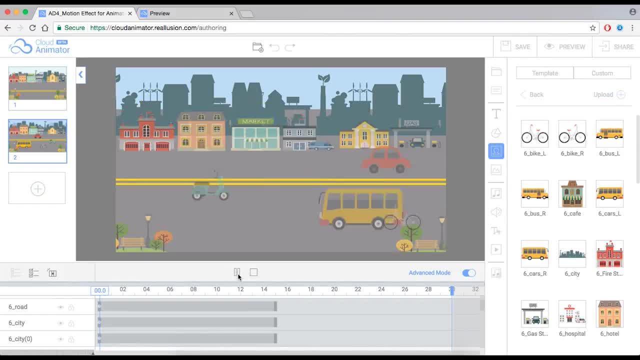 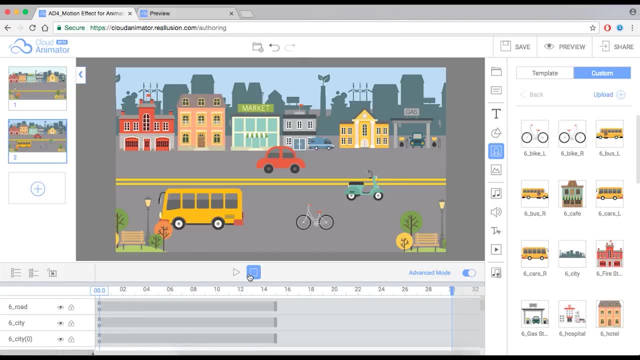 what this looks like at the end. click outside. okay, that looks okay, great. so we have our scene and we have some of these effects. but, um, let's say i wish to have these effects, uh, play in sequence. i don't want all of them to play at once, so i want them to play in sequence. so what i'm going to do? 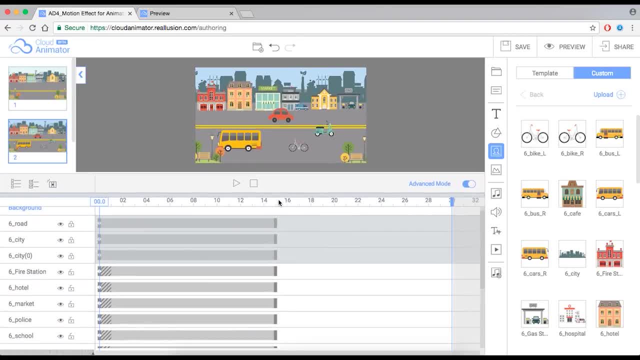 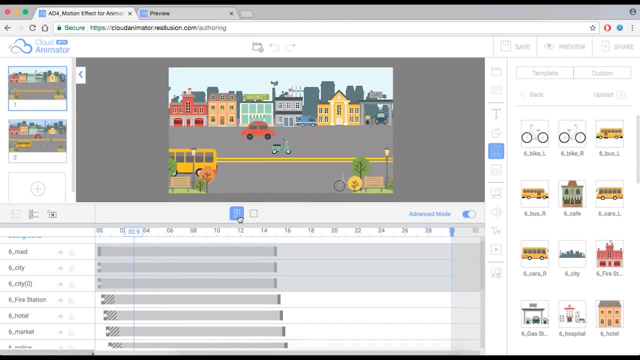 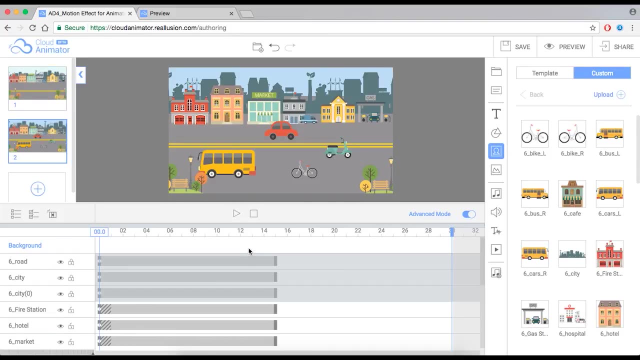 here is um, i'm going to start first with my, with my city, right with my, with my buildings. i want them to pop up one one at a time, and we do this simply by arranging that timing for each and every one. so it's very, very simple. i simply have to um, let's say, grab the fire station here, drag. 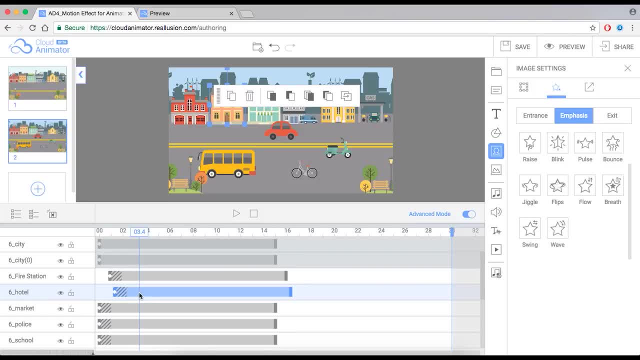 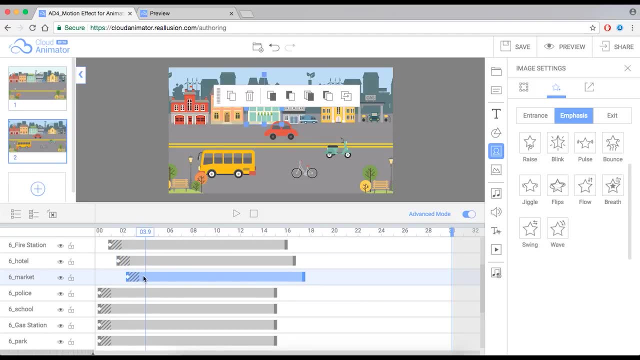 it to the right. i'll do the same for the hotel, but i'll pass the, the fire station, by, i don't know half a second or so like that, and i'll do that for each and every asset. look at that. i'll do that for the school, the gas station. 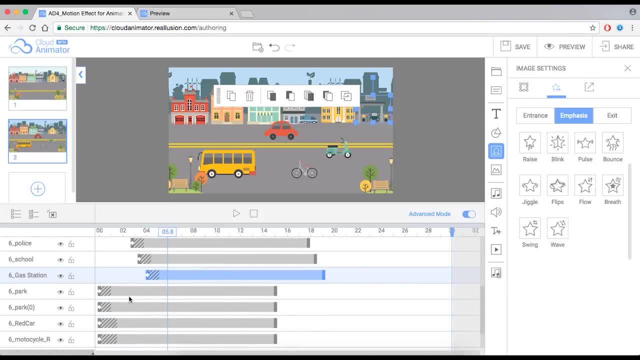 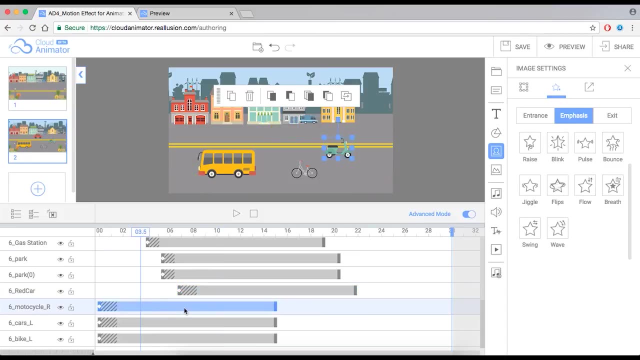 and finally the park. the park are the two parks later on, but i want these to pop up at the same time. i don't want a cascade effect. and once we have all these elements jump in, then i want the car to appear, the motorcycle, and then the bus and finally the bicycle. 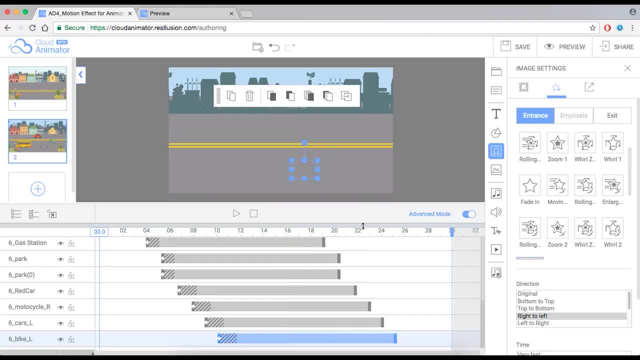 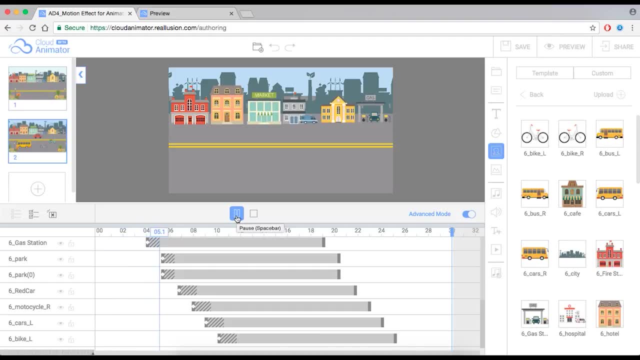 okay. so we have a cascade effect at the end. so let me play this back: we have building one, and then we have the first, okay, the park, and then wheel, motorcycle, bus and the bicycle. great, so see how simple that is. so then at the end i can choose. 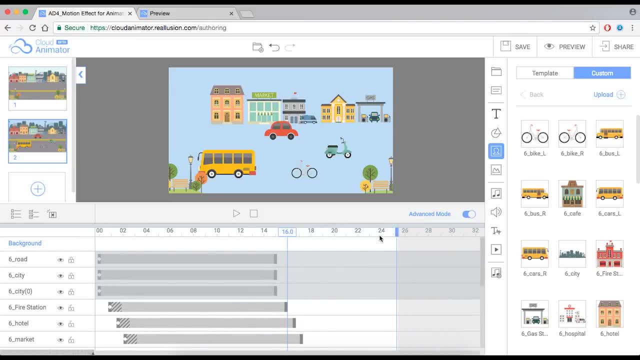 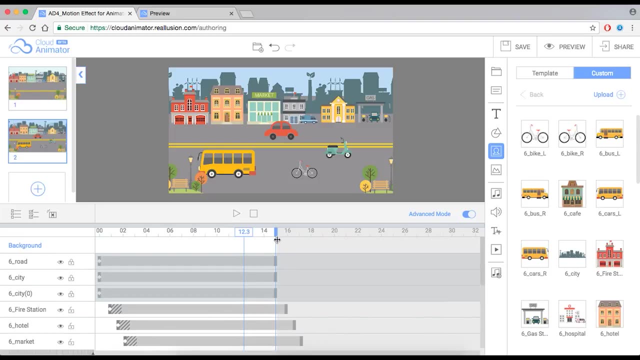 um, if i want to, how long i want my project to last notice that the background disappeared? this is because, up to this point here we no longer have, uh, that, those time tracks running, so i can basically just a side or right, i want my project to end there. that is the end limit of my project. 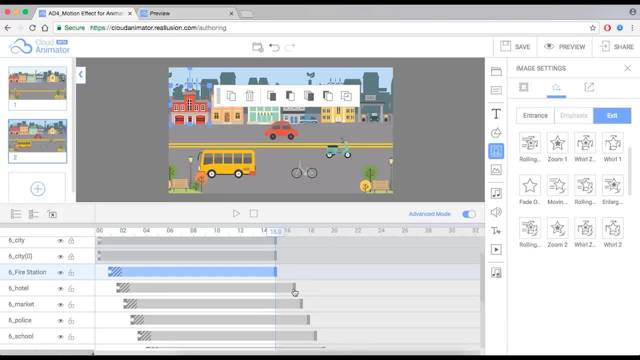 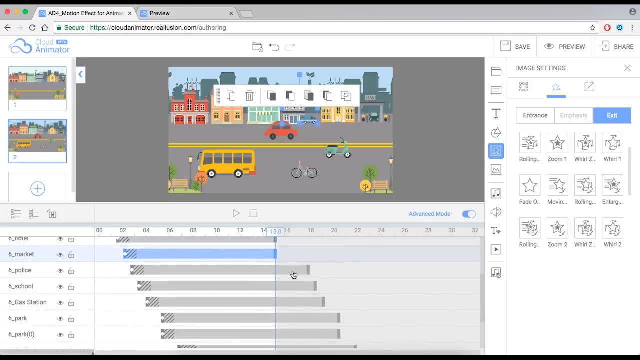 and then i can make sure that all my other elements are finishing up until that point very, very quickly like that. so you don't have to do this if you don't want, basically what? everything to start at a specific time and I want it to end in a specific time too. 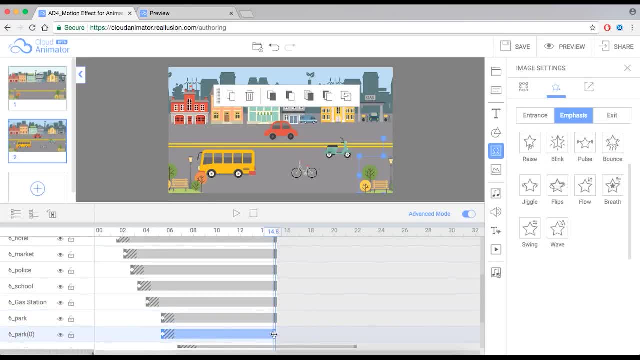 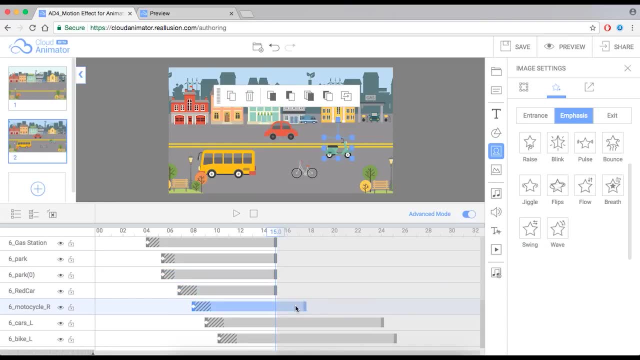 So I prefer to do this here. Of course, this is really really quickly. Imagine how long would it take you to create an animation like this in any other platform. It'll take you a bit longer, But thanks to these time tracks, you save a lot of time and obviously, thanks to all these elastic motions. 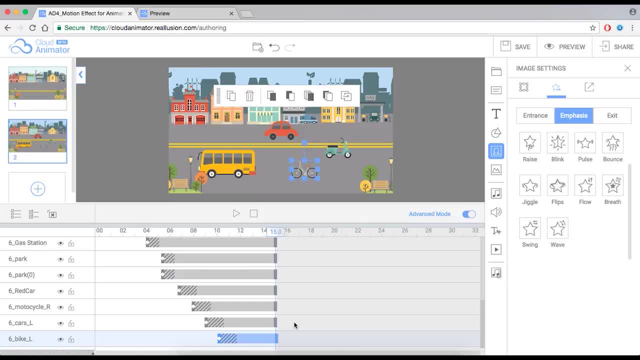 that we have here. it makes it very, very easy to not just add them, but just to manage all these projects. So at the end, let's say I want my red car to disappear, I can choose an exit And I can choose. 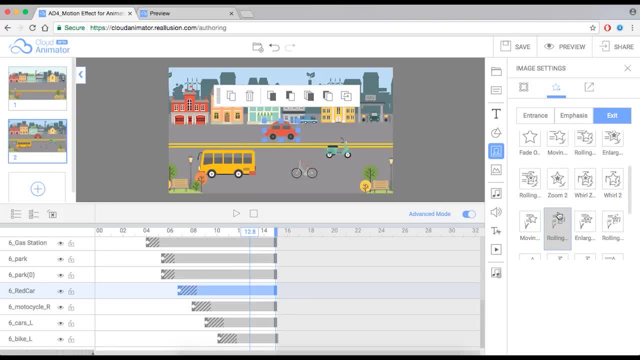 the same moving again. Let's see moving 03.. Yep, And we can have an exit And I can choose a specific place. So this one came from right to left. I can have an exit left to right, Medium speed, Okay, And I can do the same for. 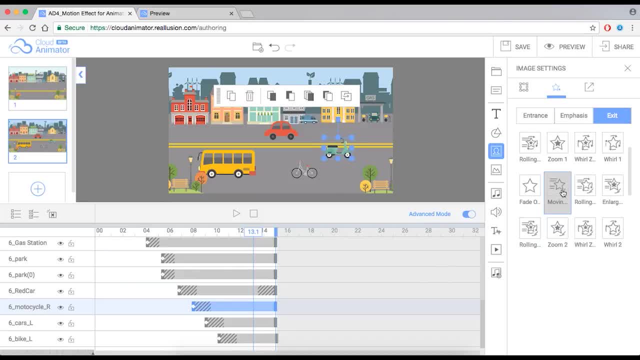 my motorcycle. This will want an exit. I want to move it. Let's say, moving Which one? The bouncy one? Yeah, We can choose that one. Was that the same one? Was that the same one? That one is called moving. 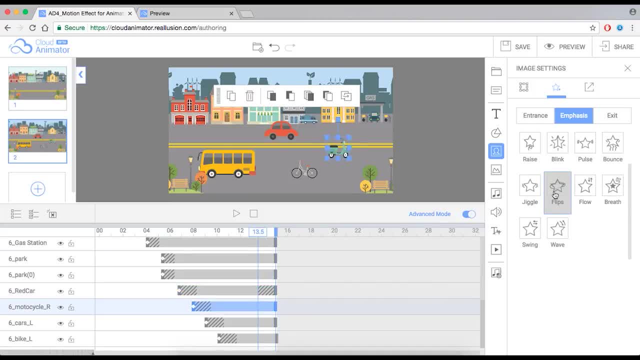 Yes, Right beside the rolling one, So I'm going to choose that exit, Not an emphasis. You need to be careful when you're selecting these, Because you want to make sure that you don't accidentally select the wrong one, So I'm going to choose that exit, Not an emphasis. 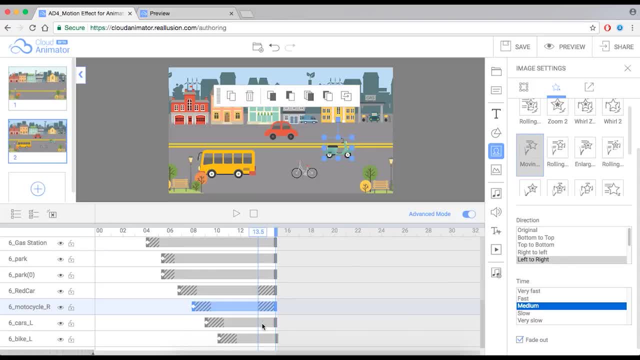 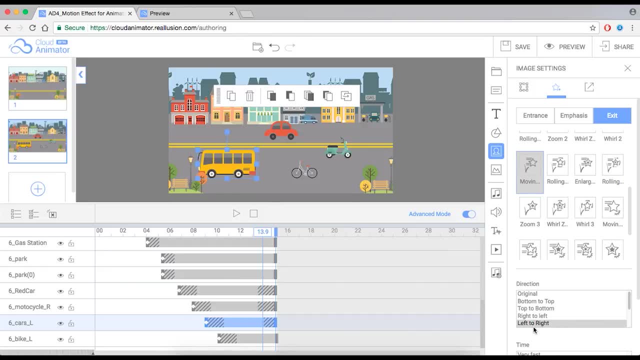 So left to right, That should be okay, Medium speed. Then I'm going to go to cars: Exit, please Moving. And this bus here, This car is going from right to left. That's the way I want him to exit And then